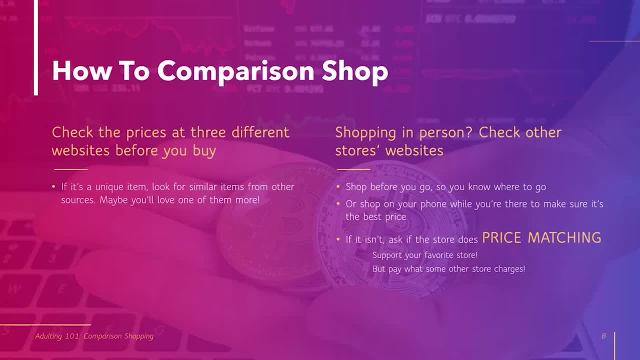 comparison shop. Well, that's what we're here for, right. If you're comparison shopping online, it's a good rule of thumb to check the prices at three different websites before you buy. The same thing is actually true if you're buying an item that you can only get at one place. It's a good idea to. 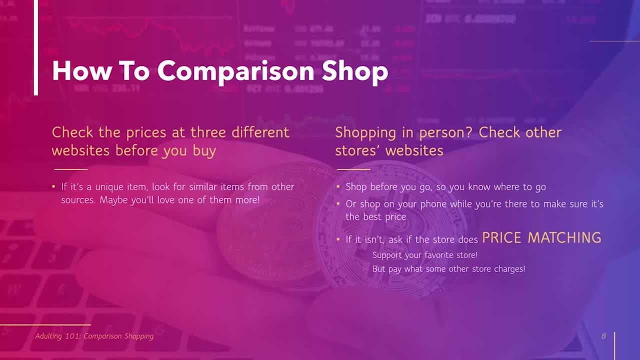 look for similar items from other sources. That way you'll get an idea whether the price is really appropriate for the quality you're getting. or, who knows, maybe you'll find something else you even like better. Now, if you're shopping in person, check other stores' websites If you. 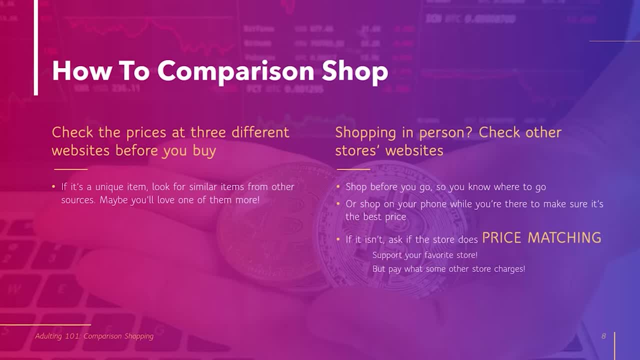 shop. before you go, you will know what store to go to. If you shop on your phone while you're in a store, you can make sure it's the best price and if it's not, you can ask if the store does price matching. that's when you prove that the stores competitor has. 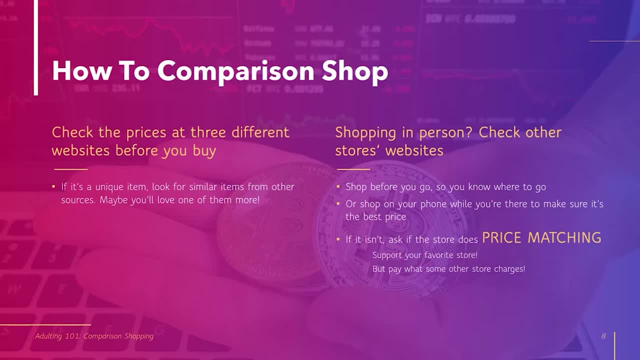 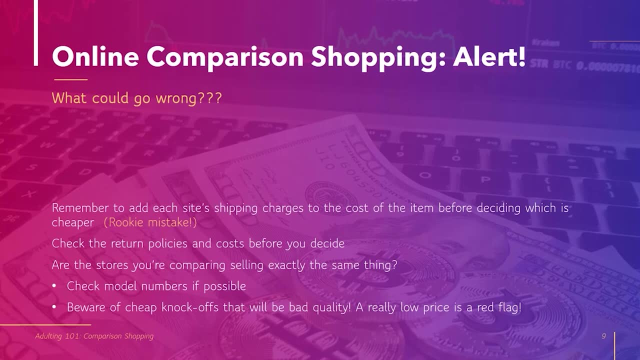 exactly the same item for a cheaper price, and your store honors that lower price. so when you're shopping online, what could go wrong? first, don't make the rookie mistake of forgetting to take into account each sites shipping charges. you don't want to save five dollars by buying from one site only to discover 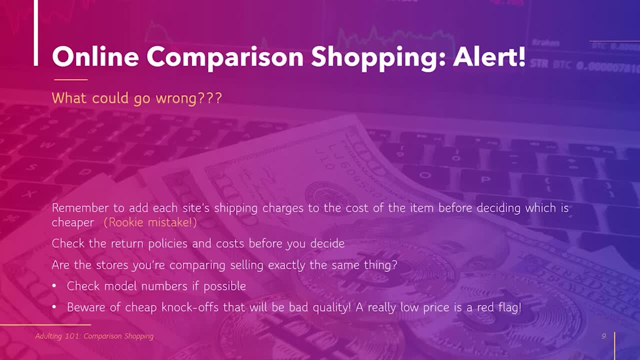 that the shipping is seven dollars when it was free on the other one. another thing to consider is: are the stores you're comparing selling exactly the same thing? if you can check model numbers, that's a good thing, and if you're noticing a really low price, that's a red flag. beware of cheap. 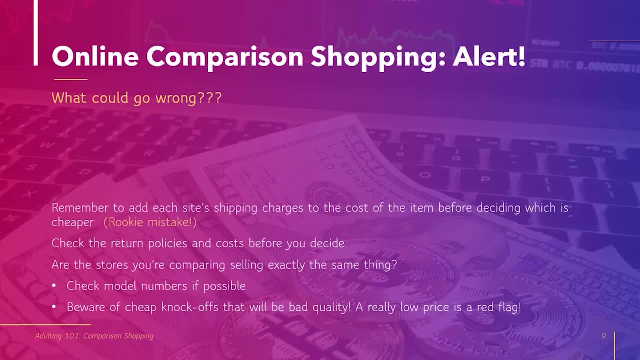 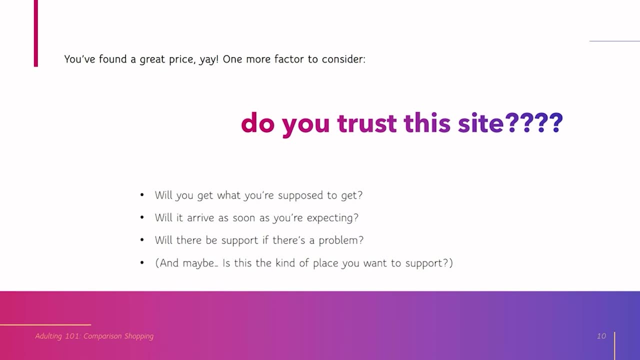 knockoffs that will be really bad quality. or consider whether you're not getting the actually actual thing but just like an accessory for it so you found a great price, go you. one more factor to consider: do you trust that website you're buying from? do you think you're gonna get what you're supposed to get? will it show up when? 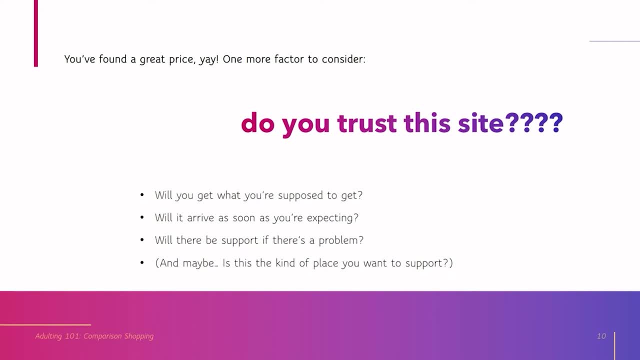 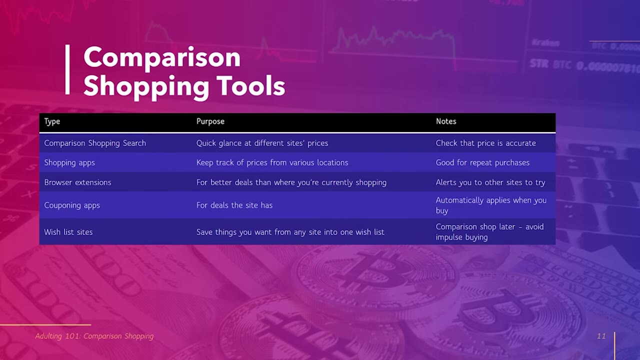 it's supposed to? what kind of customer support is there if there is a problem? and also, is this the kind of place you want to give your money to? you might have ethical or political reasons to boycott or favor companies. so here's, here are those comparison shopping tools I mentioned earlier. now I don't want to. 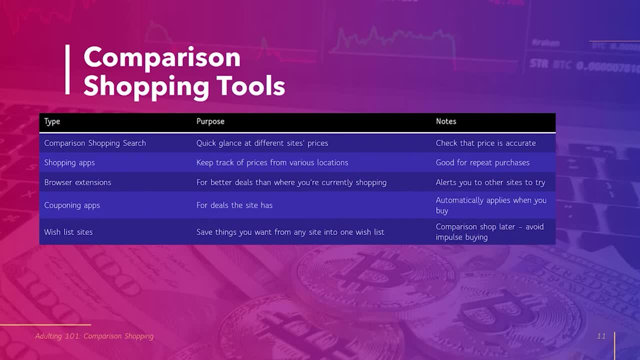 recommend particular products or sites but, knowing these exist, you can go search out the things that are going to work for you. first up the comparison shopping searches or websites. this gives you a quick glance at what a whole bunch of different people charge for the same item. now you do need to click through to 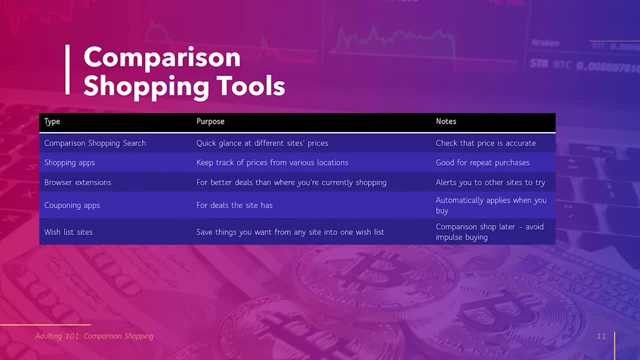 make sure that that price is accurate, because sometimes the feed can be off. it's very important, I think, for you to go and get yourself a shopping app. it helps you keep track of prices for our different items from different locations. just do a quick search in your App Store. a lot of different apps have different 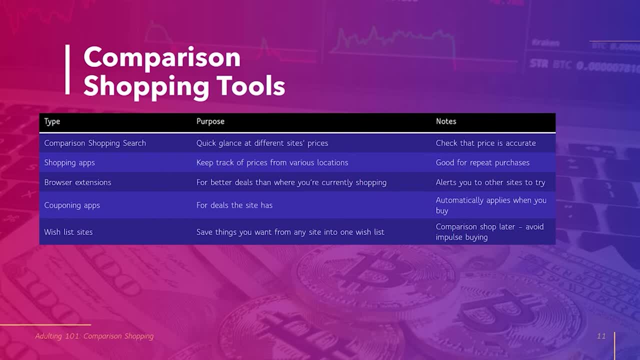 options and you can pick something that really matches what you need. I want to make sure that you know that there are browser extensions. if you're shopping on a laptop, if you're shopping on one particular site, it'll just pop up to let you know that hey, there's another site out there. 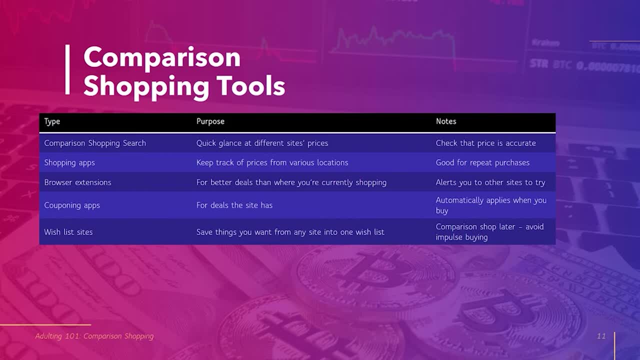 you're shopping on a laptop. if you're shopping on one particular site, it'll just pop up to let you know that, hey, there's another site out there there that has it for a lower price. That can really save you some time and brainstorming who to look for. There are also couponing apps that you can just have running in the 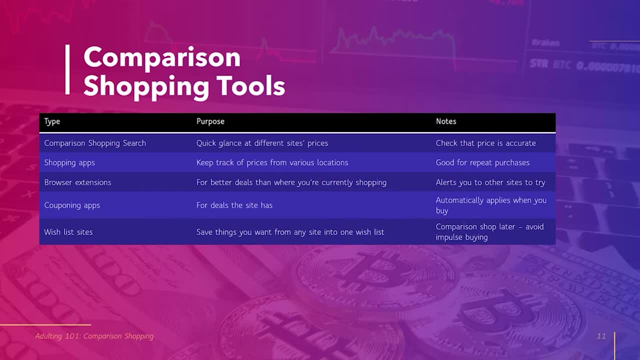 background. This is kind of nice. when you actually go to buy something, it will automatically apply any coupons it can locate for that particular site And finally get yourself a wish list. Now, okay, you probably have like an Amazon wish list or wish lists at a lot of different. 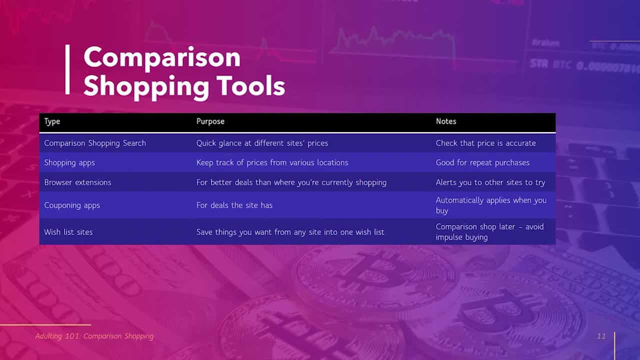 places, but you can get a site that holds your wish lists for every website you visit. Save everything you want. Now, how does this save you money? Because it keeps you from impulse buying, If sometimes you're afraid that you won't ever find this thing again. 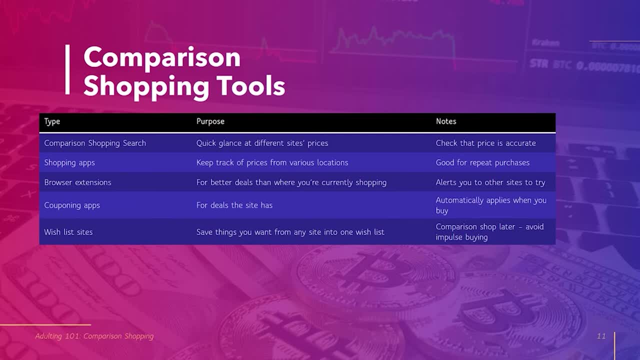 put items that you like into this wish list site and come back later when you have a cooler head or when you have more time to comparison shop, And that way you won't end up filling up your room with stuff that you loved for the first day or 30 minutes. 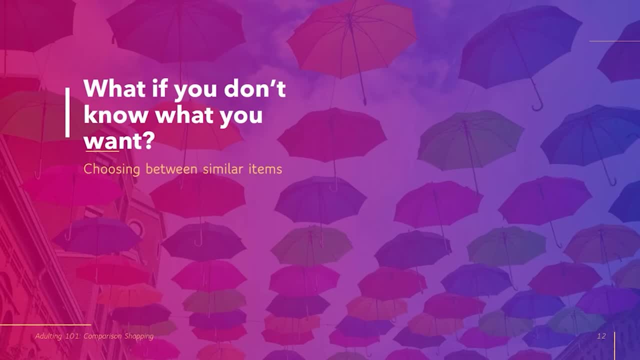 Okay, And then didn't actually care about having. But what if you don't know what item you actually want? So I would love to talk about how to make decisions, but that's really too big for this video, So I'm going to give you just this one tool If you regularly use.